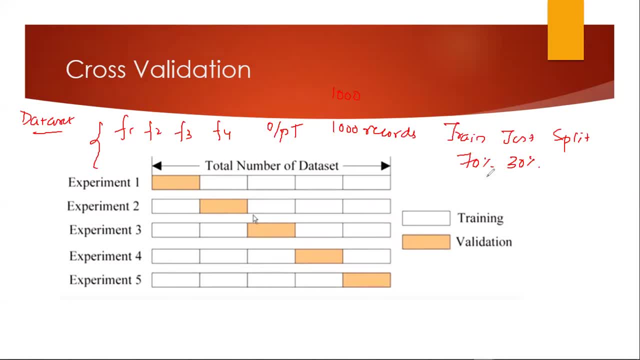 data set, that we have, number of records that we have. Now, when, when we do this strain test split, then what we do is Is that we give the 70% of our data set to our model. model gets trained with respect. 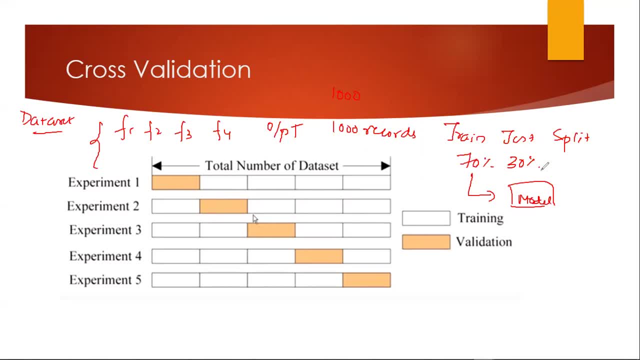 to our input and output feature And then, once the model is getting drained, after that we test this particular model. We test the accuracy of this model by giving the input of the remaining test- 30% of the data, And then we see the output And then we try to. 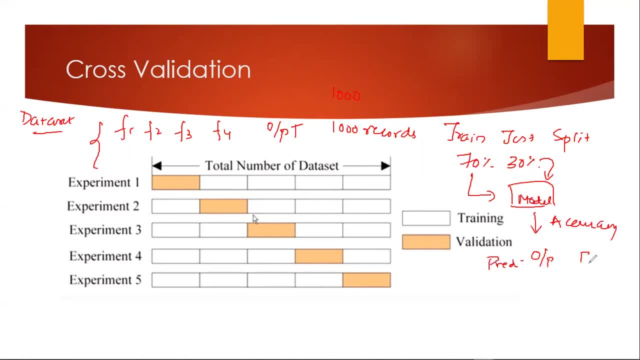 verify this predicted output will with the real test output. right, With the real test output. Now, when we see this particular output, suppose we have this particular output, We have this particular output, We have this particular output. Suppose I'm getting my model accuracy is giving somewhere around 83%. Okay, Now 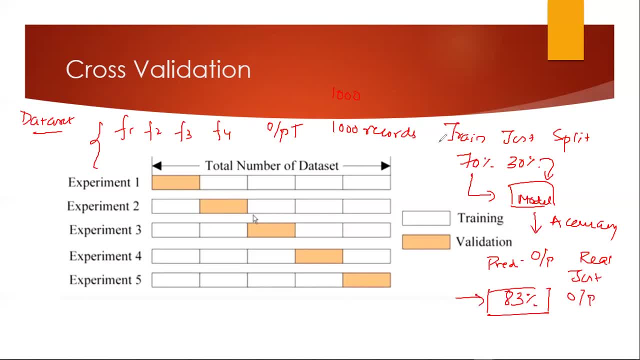 when, when, when we get this particular 83%, it is with respect to one type of train and one type of test data. Now it may so happen that the 70% of the train data and the 30% of test data- some of the reports- may come over here also in the next iteration, Suppose. 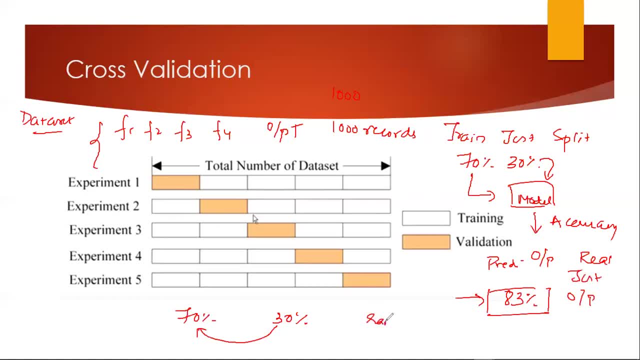 I want to do a separate train test split by using a different random number variable. Okay, There is a parameter inside train test split which is called as random number And suppose if I give a random number of something different and that and what happens is that it again randomly picks up some other 70% of the data. 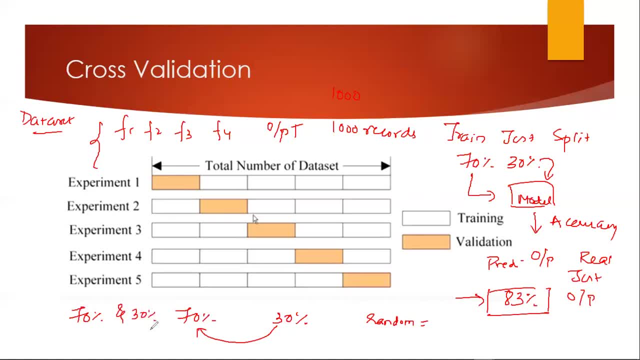 as my dream set. And then I uh, then then the test data is the remaining 30% of the data And it randomly picks up, it shuffles the data set and randomly picks it up. Now, at that time, when I give this kind of data again to my model, then the model may be giving 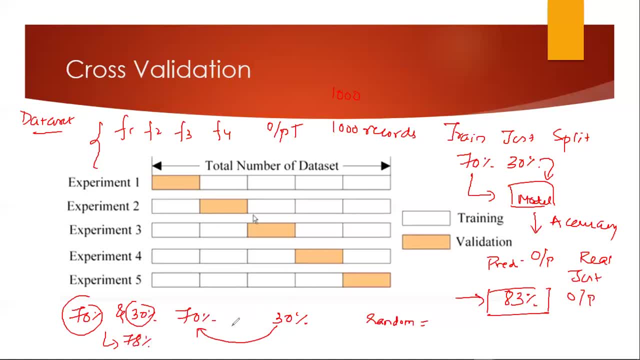 my accuracy somewhere like 78% or it may also increase or decrease based on the train type of data. that is basically selected in my training set and uh and the test set. So this random number shuffling and the train test split actually works for one type of 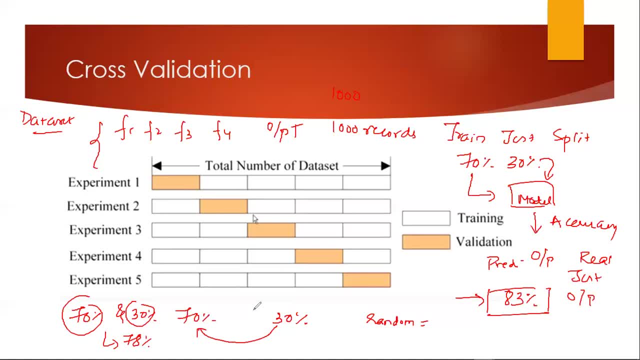 data itself. It is a. it is a. it completely depends on what kind of data are basically on the 70% of the site, what kind of data are basically on the 30% of the data. Now, imagine that we should try to know in order to prevent this, like every time we are shuffling. 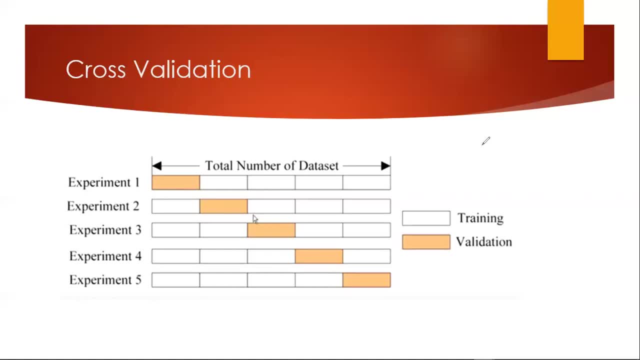 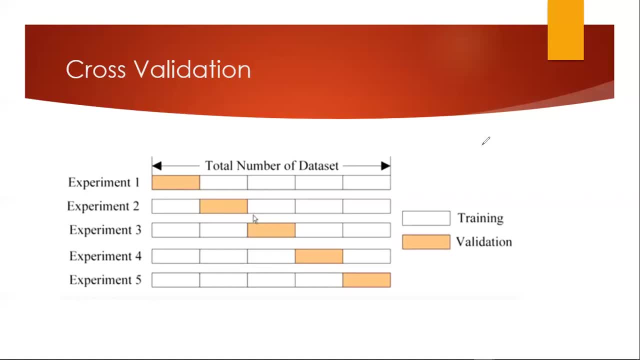 purpose right All the time will be getting some different accuracy, So we will not be able to, you know, come to a frequency parameter that what is basically the accuracy of the model by just seeing one type of plane, and so because of that, we basically use something. 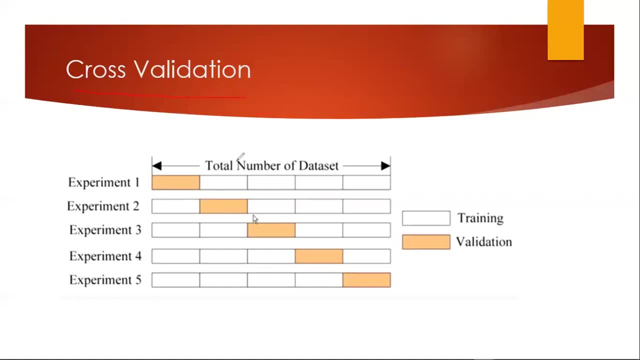 called as cross validation. Now, the cross validation works somewhere like this. Now let us consider: I have total number of records That's 500.. So 500 is my data set, Are you? I try to divide this. okay, now, I'll be considering that. let me consider 450. 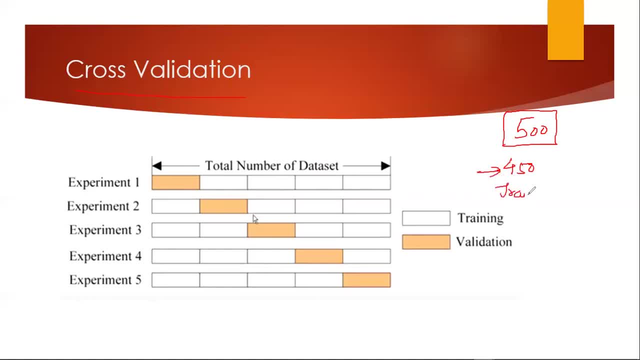 data set for 50 record should be always in my training data set and then 50 record should be always in my test data set. this is basically test accuracy. okay, now what happens is that cross validation works in such a way that suppose I'll take this 500 data set again and I know that I have to have 50. 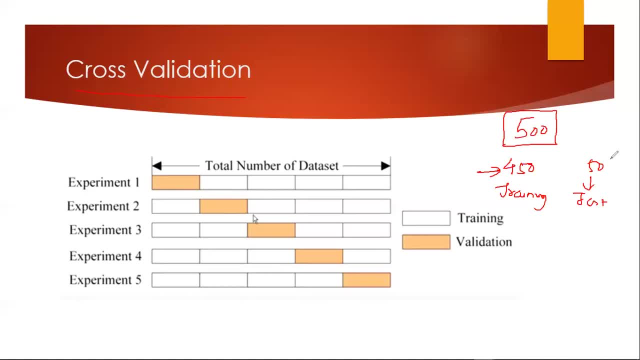 tests it test: 50 data set in my test, so 50 records in my test. so what I do is that I will take all this 500 data set once in this particular square box. let me just take the first 50 data set as mine as my test data. okay, now the 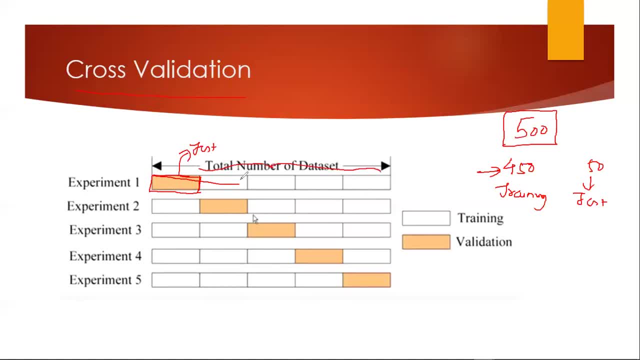 remaining 450. what I can do is that: okay, remaining 450 now. okay, I will not consider 450, because I've just made five groups. instead, what I'll do is that if I'm taking 500 as my total data set, then what I'll do is that 400 I'll keep it in my train. 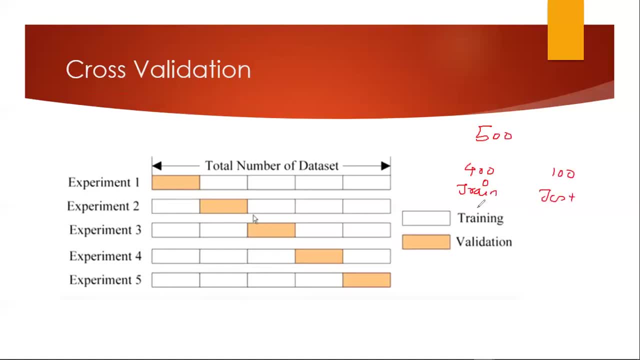 and remaining hundred. I will be keeping it my test. okay, now I can divide this into five different experiments. in the first experiment, my first hundred records will be my tested data set and then the remaining data set that I have. this will actually become my trained data set. okay, now, always remember, see. 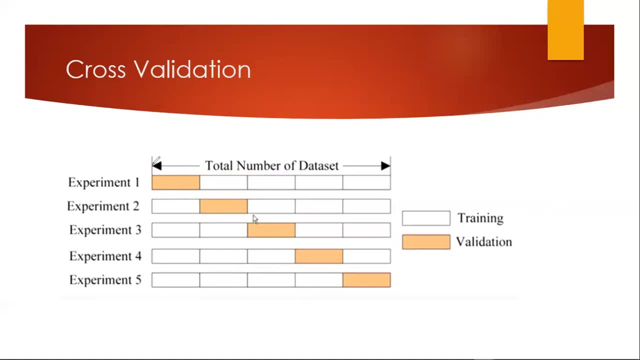 how, how, how. the cross validation will happen in the first iteration, I'll lateration my first record, first known, that record will basically my test and remaining all will be my training data. now what I'll do: I'll take this data set, I'll give it, I'll train it in my model, I'll I'll take. 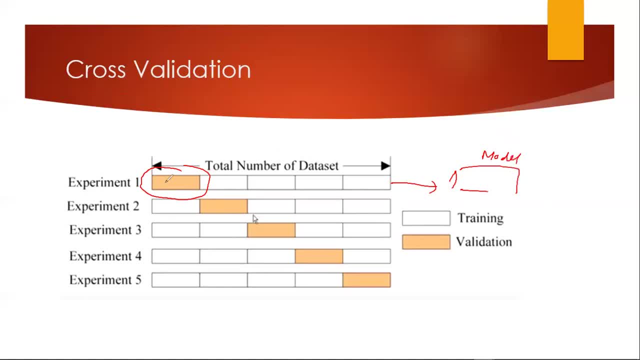 this training data set of 400 over here, give it to my model and then test with this remaining test data and get one kind of accuracy. so this will be my accuracy one. similarly, what I'll do is there in my second experiment. I'll just move towards one, a heart step. that is my next 100 data set, which will be my test itself. 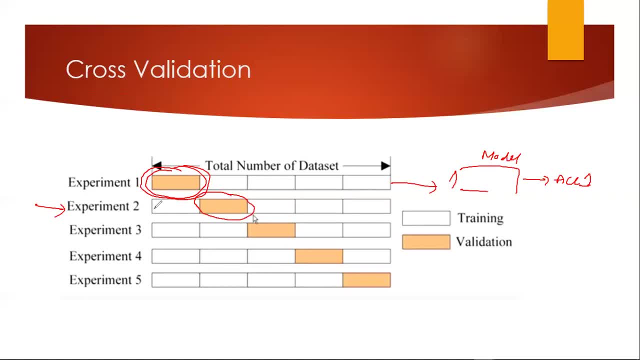 set over here. I will consider this as my test data set and remaining data set will be my training data set. then I will give it to my model. okay, my model will get trained and it will give me another accuracy. similarly, what I'll do is that I'll complete this iteration for all the experiments. 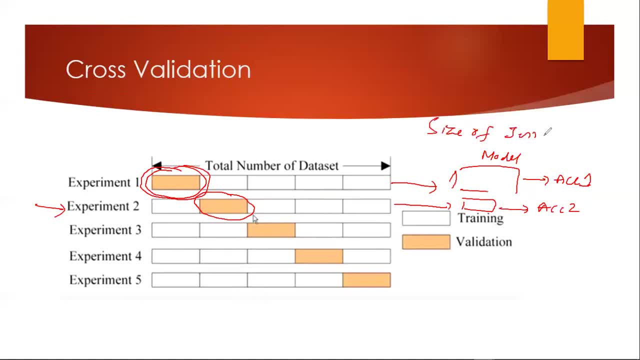 based on the size of the test data. now why I'm saying based on the size of the test data. where I've taken my test, data size is 100. so if the total number of records are basically 500, then what will happen is that the first iteration I'll get 100. remaining 400 will be my training data set. 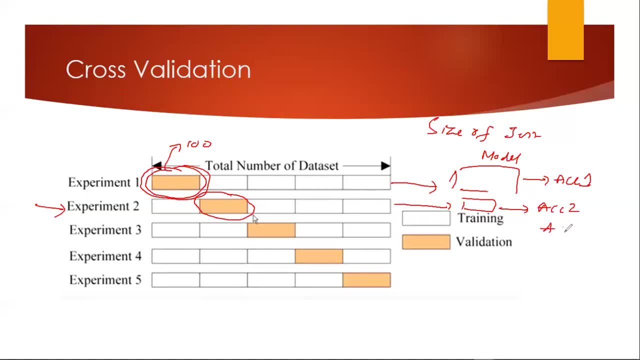 similarly, I'll complete all the iterations. then I will be seeing that based on the number of iteration, I'll be having that many number of accuracy. so here I have five iterations. I'll have accuracy one, accuracy two, accuracy three, accuracy four, accuracy five. now, since I am having 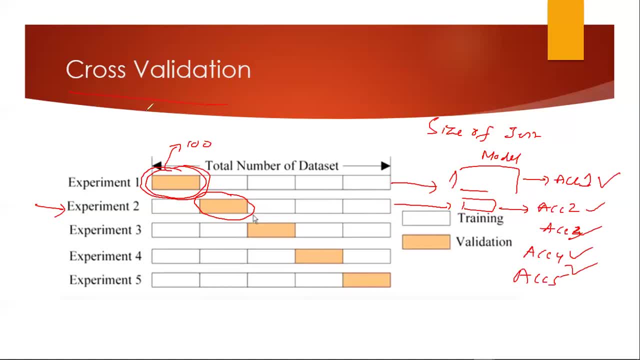 different accuracy. what my final cross validation will do is that it will try to find out the mean of all this accuracy, mean of all this accuracy. now, when I find out the mean of all this accuracy, this will then be giving me accuracy which is actually, which is actually representable for the complete data set, wherein you're shuffling the data and you're 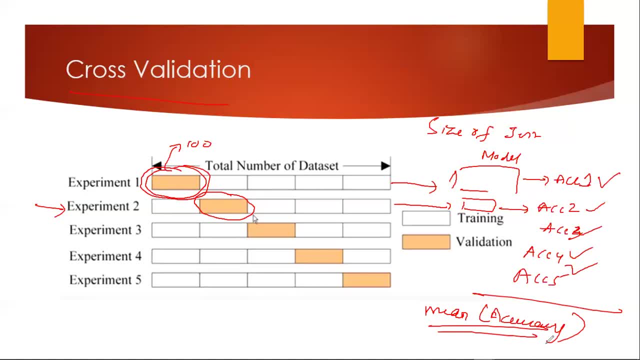 trying to take it as a train and test, so it is actually using different train and test data and actually calculating your accuracy. and this is how a cross validation work. simple guys, serious. in the first experiment, what I'm doing, I'm just considering that my top 100 record will be my test data set. 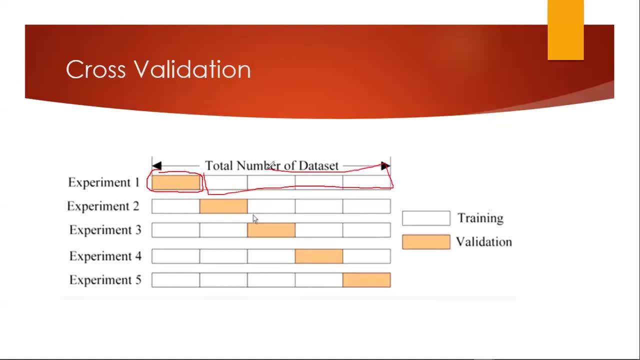 remaining, all remaining, all this will be my training data set. right now, I'll give it to my model, train it, and this will happen for all the experiments. now, how many number of experiments will be there, based on how many number of records I have right, and then how many data set I'm taking it as my test data? 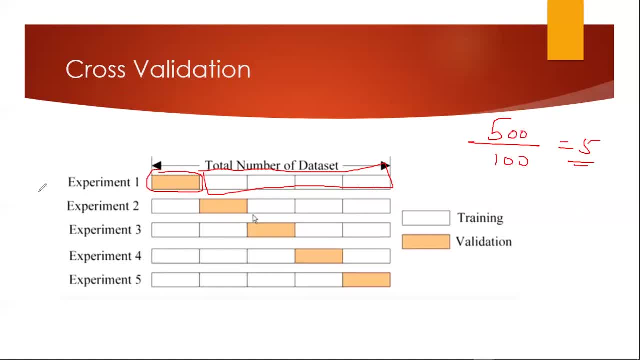 set, 500 divided by 100 is nothing but 5. so this will actually be 5 experiments, you know, and based on this, what will happen? every one, every experiment, will have different, different accuracy. then, finally, all this accuracy mean will be- we will be calculating mean of all this accuracy will. 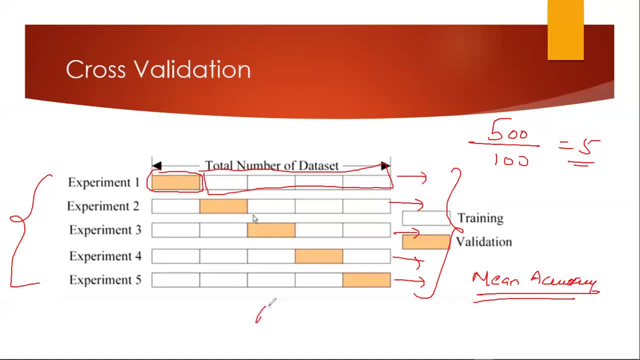 we will be calculating and finally we get the type of accuracy that is representable for the whole data set and this is pretty much pretty much good and pretty much valid when compared to the train and test train and display and sometimes cross validation also helps you to choose like what algorithm you should use, how I'm saying that, suppose. 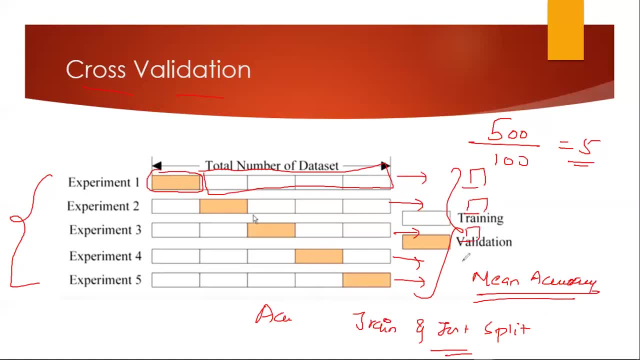 you are applying logistic regression over here for all these particular experiments, okay, and then in the second time you apply decision tree. now, suppose your logistic regression average is coming somewhere around 68% accuracy, the decision tree may give you an accuracy of 73%, right. so how do you choose this algorithm? by select, by seeing the cross validation score. 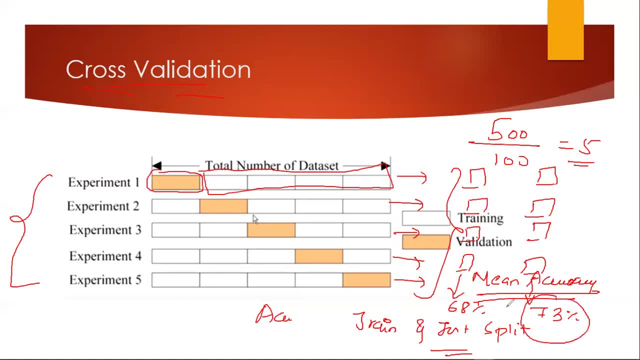 that is your mean accuracy of 73%. this is much more better than the 68%, so you may choose decision tree for this particular problem statement. Similarly, you can apply it for other other types of algorithms. and this was all about cross validation. guys, I just also help you to see a coding functionality. just give me. 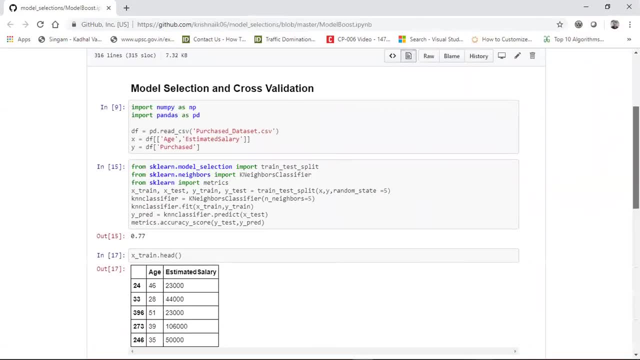 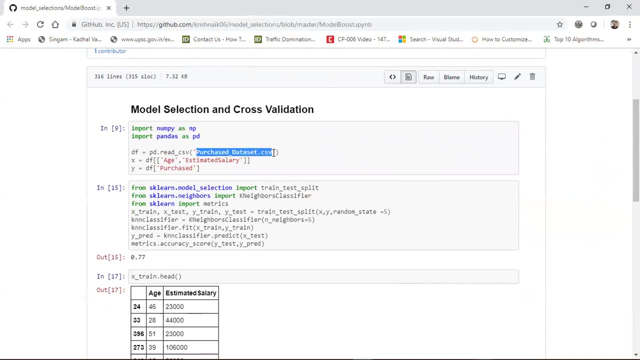 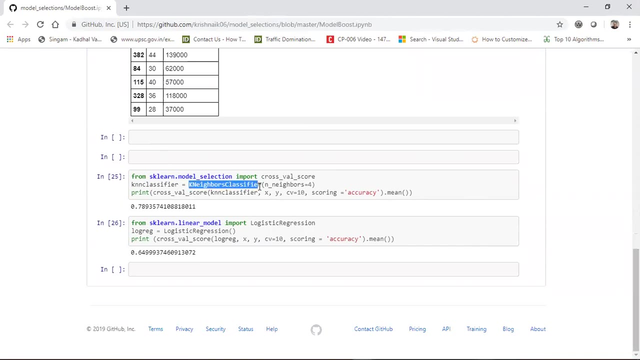 a second. so here I have actually made a Jupyter notebook file of model selection and cross validation. here I've considered a data set which is called as purchase data set, dot, csv, and here you can see that after applying I'm trying to see with K near, near, K, nearest name. 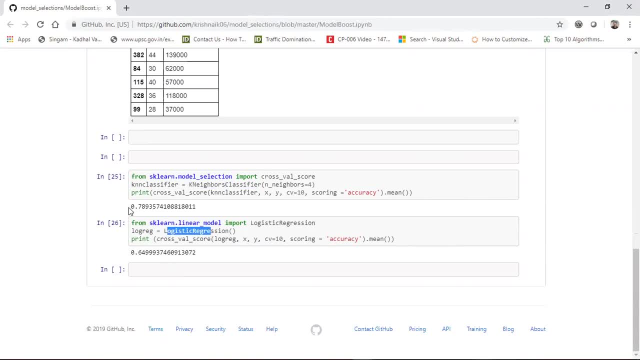 equals classifier and logistic regression. you can see that after applying cross validation, I get a mean score of 78% and the mean score of 64%. you can go through this particular file. I'll provide this in the this already uploaded in the GitHub link. I'll provide the. 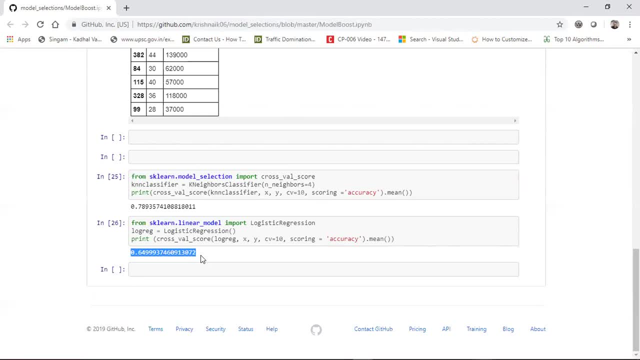 link in my description of this particular video. I hope you particularly. I hope you like this video. guys, please make sure that you subscribe to the channel. thanks for supporting everyone. please share with all your friends. I do come up with very interesting content and I'm pretty much sure that I'll come again with much more interesting content. 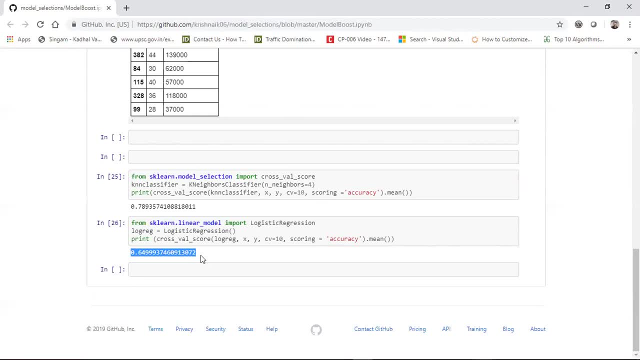 Thank you for watching. Watch more contents in my next videos. Thank you one and all. have a great day. Thank you.